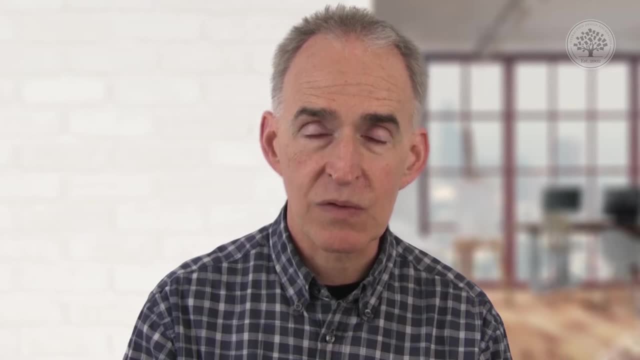 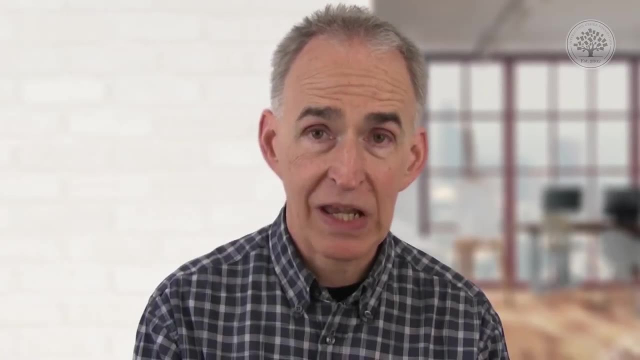 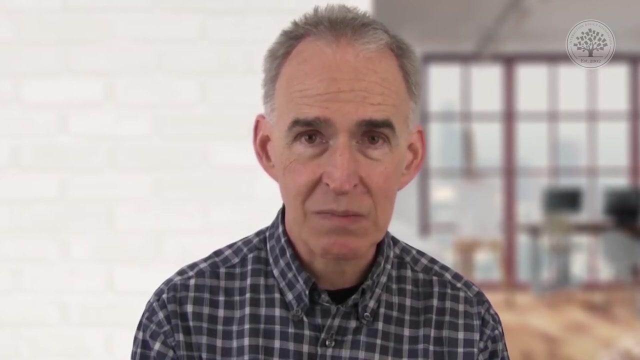 individuals rather than groups, And I will be back in just a moment. The general feeling is that when we dehumanize people by referring to them with these abstract collective nouns- because collective nouns are abstract by definition, So we're talking about users or we're talking about customers- We're taking the people away. We need to put 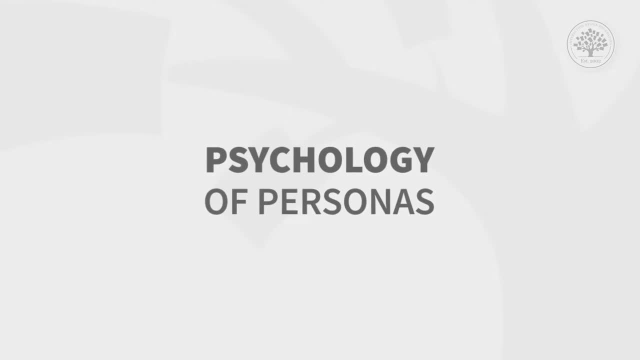 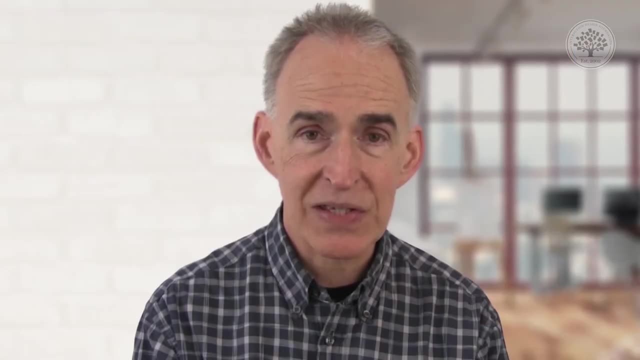 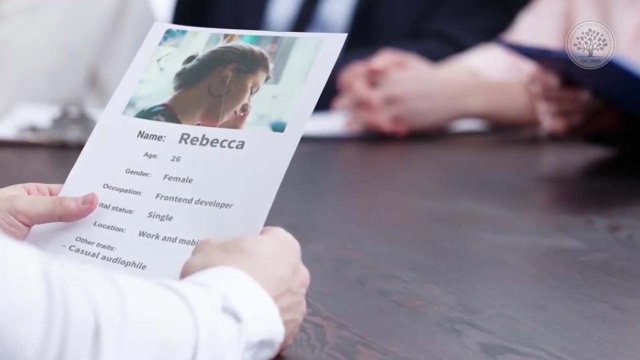 the people. back Back in 1983, David Sears ran a study with two sets of participants. He gave the participants the same characteristics And in one set of participants he said that these characteristics were of an individual and I believe he described the individual. And in the other set of participants he said 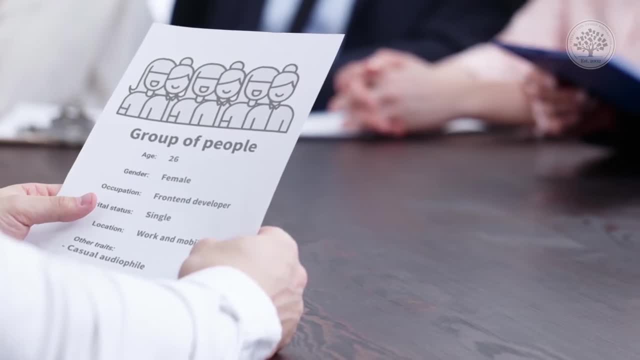 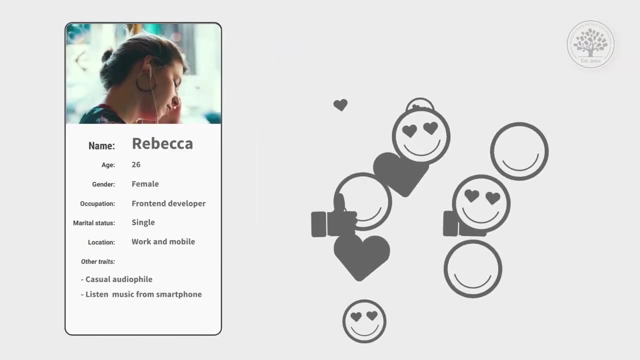 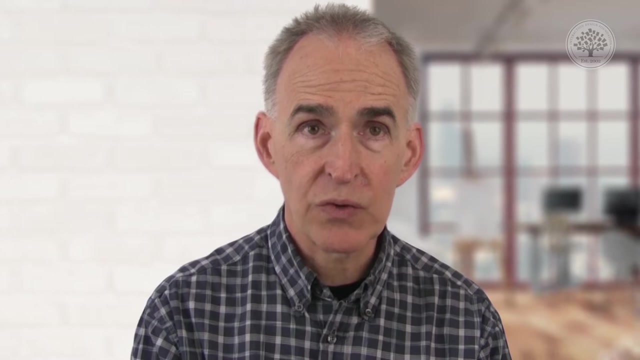 that these characteristics were of a group of people And the participants who were told that they were seeing the characteristics of an individual always rated the individual more highly than the participants who rated the characteristics in connection with a group, So that he called the person positivity bias. And it is not necessarily true, because we're 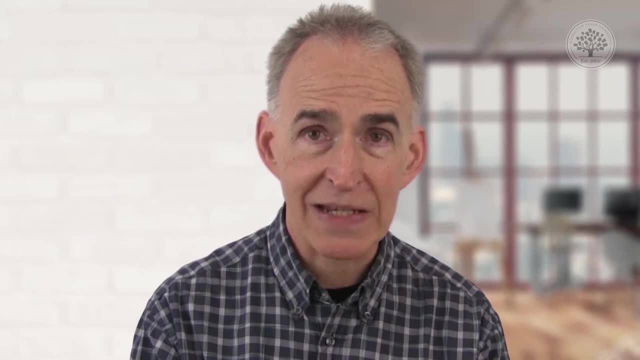 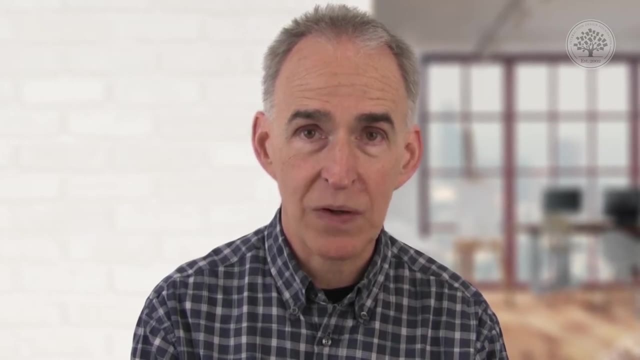 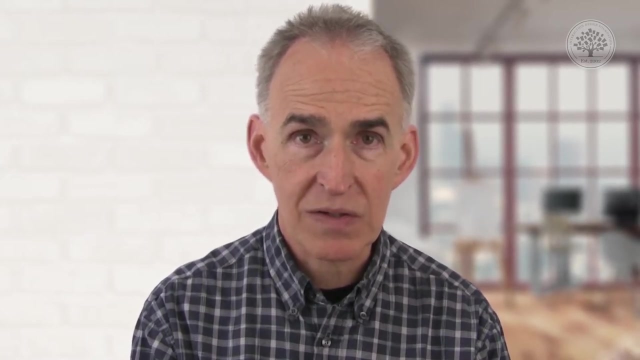 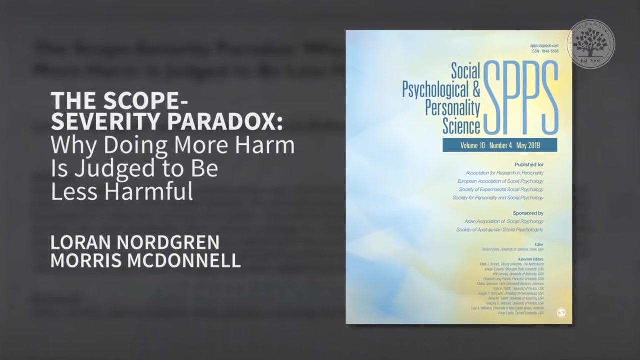 basically is confirmation that our brains are us as individuals- prefer thinking about other individuals- certainly more inclined to think more positively about other individuals than we are about collective nouns like tourists or customers or users. the scope severity paradox is a much more recent piece of work- 2010- and is quite surprising in two researchers, north green and mcdonald. 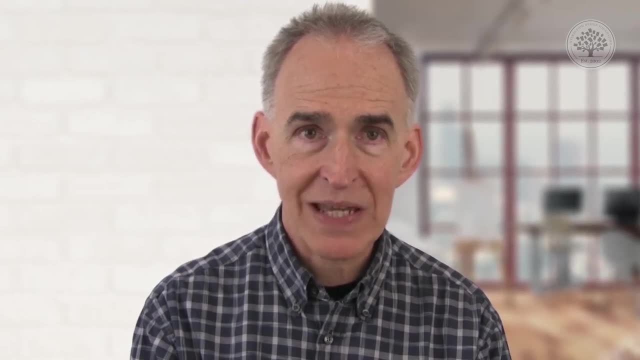 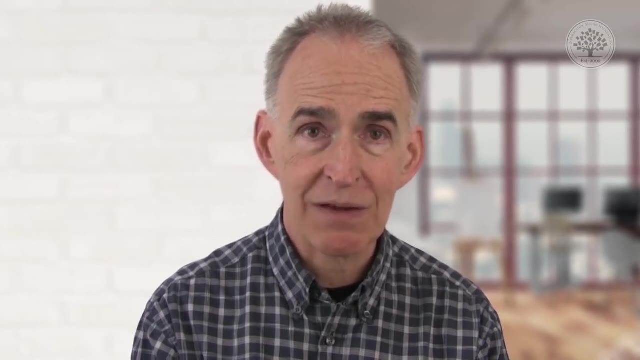 established that reactions to a fraud were more severe when it was presented with three victims rather than 30. so it's the same kind of deal: two set of participants both given exactly the same details of a crime, except that in one group. they were told it. 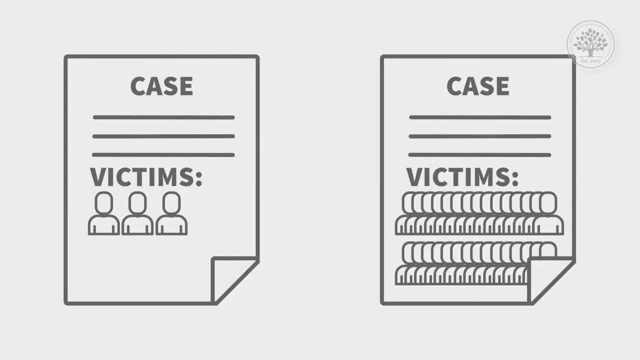 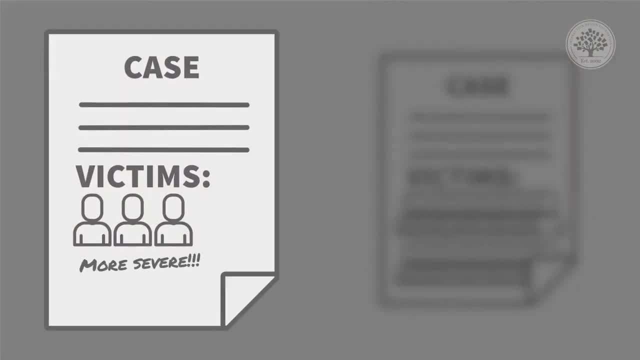 affected three people and the other group. they were told it affected 30 people and it was the people who were told that there were only three victims that thought that the crime was more severe and they, on average, added a year on the prison sentence that the perpetrators of this 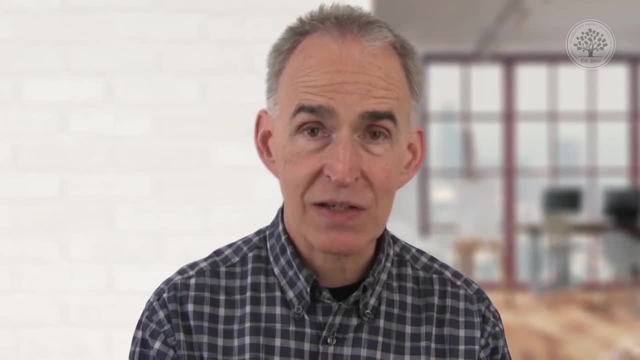 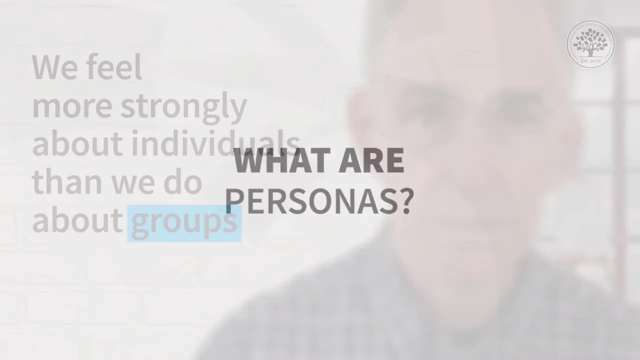 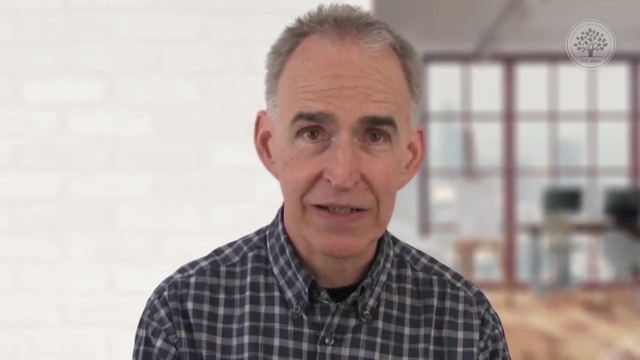 crime should receive. so again, that is just confirming this tendency for us to feel more strongly about individuals than we do about groups. personas are fabrications based on research. we mustn't let go or lose sight of that little parenthetical expression there, because we go out and we find out. 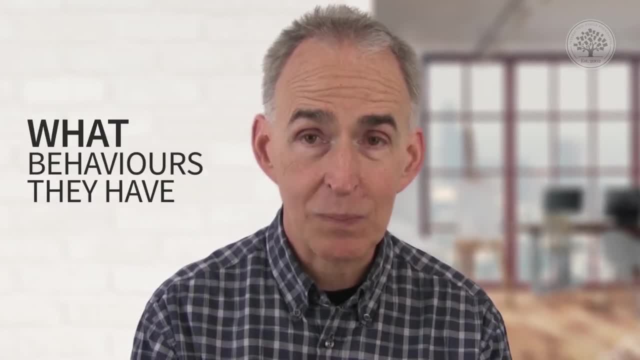 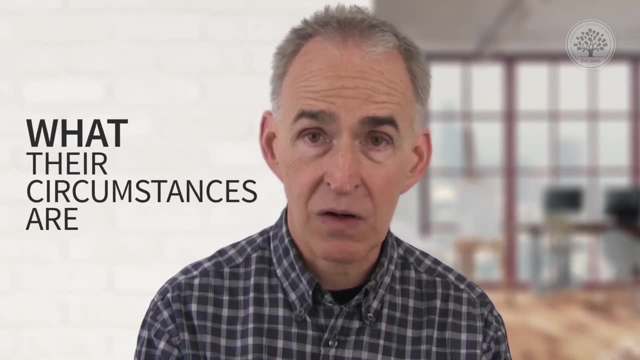 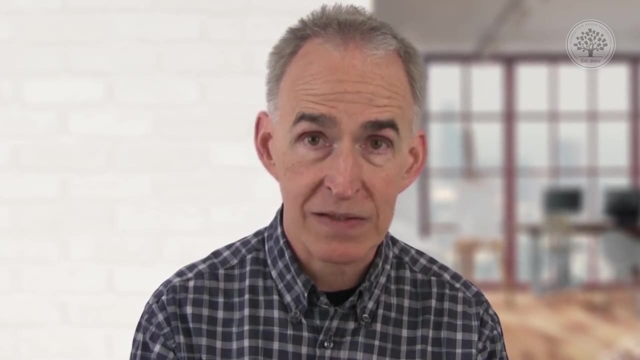 who these people are, the ones that we're interested in find out what behaviors they have which drive them to need our solutions, what motivations, what their circumstances are, what their the contexts of use are, just so we understand who we're building the solution for and other aspects that we describe in the context of. 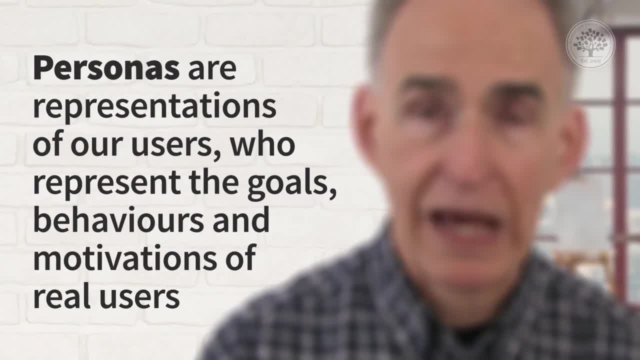 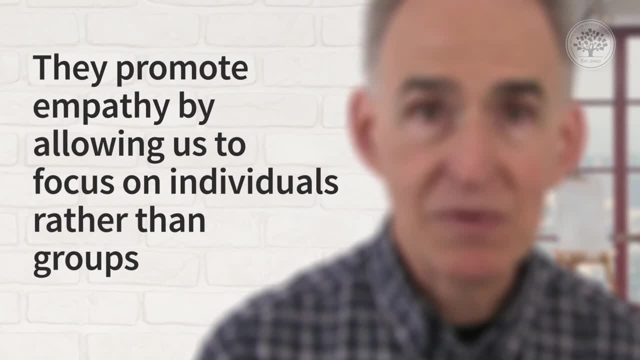 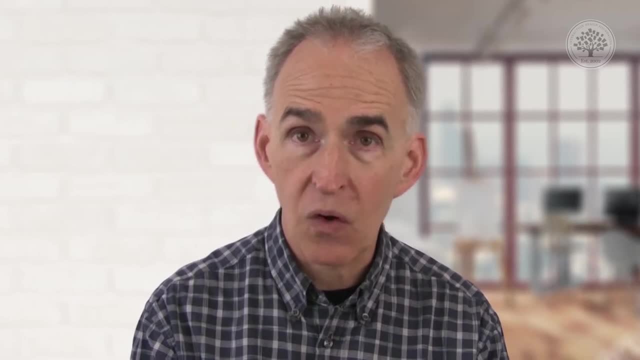 use. these personas are representations of our users, who represent the goals, behaviors and motivations of those real users. they promote empathy by allowing us to focus on individuals rather than groups. so, instead of talking about user community one or whatever we're talking about- whatever catchy name we'd like to come up with for our user communities- we start talking about. 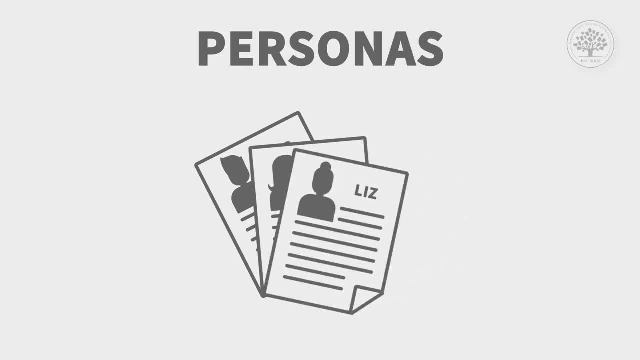 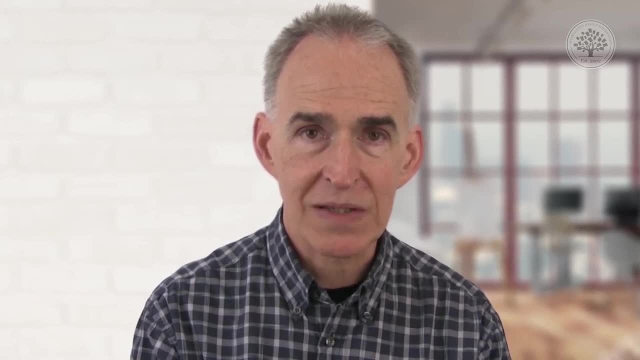 bob or jane or elizabeth, whoever, whatever everybody in the team is happy with, and there have been all kinds of documents and papers and studies written about personas and you'll find that personas range from quite a limited description of a person and in fact it can be just as little. 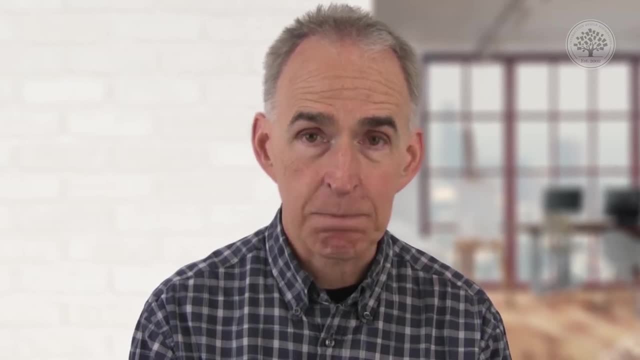 as changing the name users to a certain description of a person or a group of people to be able to to a person's name. So if you always referred to your customers as Andrew, then you would actually be doing yourselves a favor in terms of making that customer seem much more real. 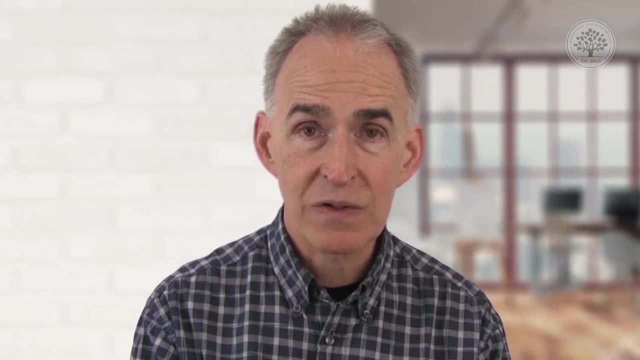 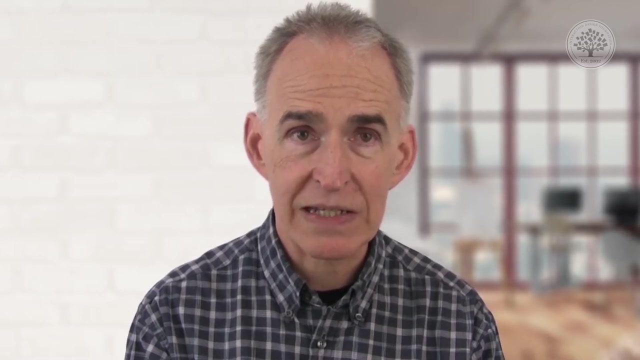 But, at the other extreme, it's not uncommon to hear about user research and persona development taking weeks, possibly even months- two to three months, which is, in my view, and quite a few others certainly, for an Agile environment- well beyond the realms of possibility. 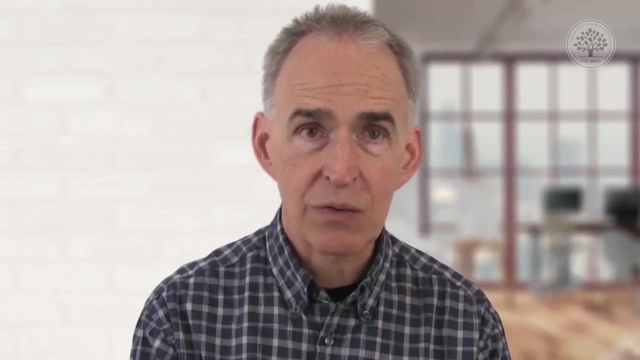 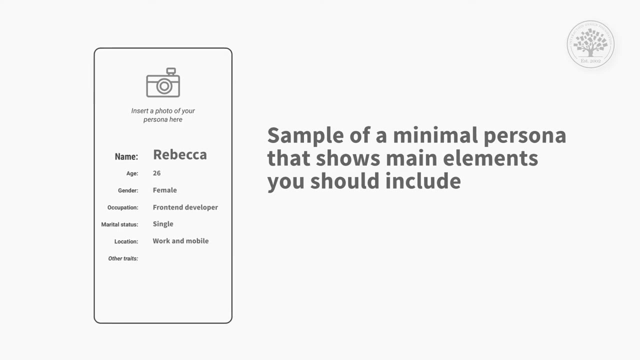 So we're gonna be talking about something called a minimal persona. So minimal persona- a name, age and other specific demographic details- that a real person would have A photo- ideally realistic- showing the person in that setting or doing that thing. 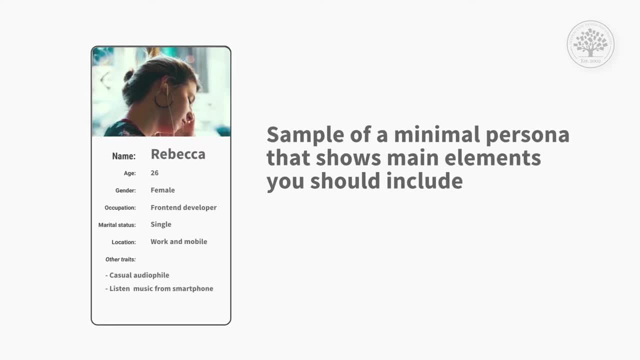 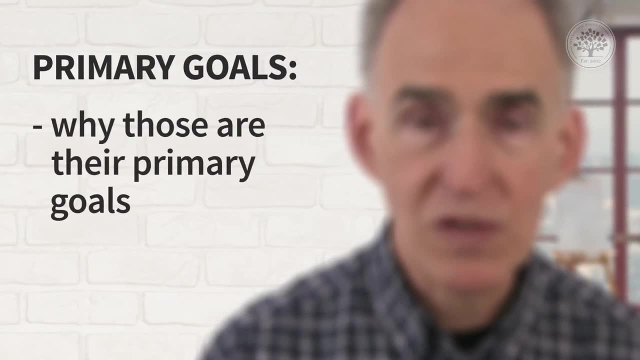 and then basic information about why you're interested in them or why they're interested in us- our solution or product, So their primary goals, why those are their primary goals and what they're hoping to achieve through our solution or product and their behaviors. 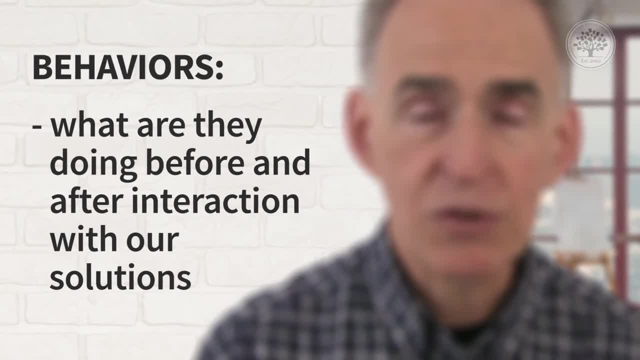 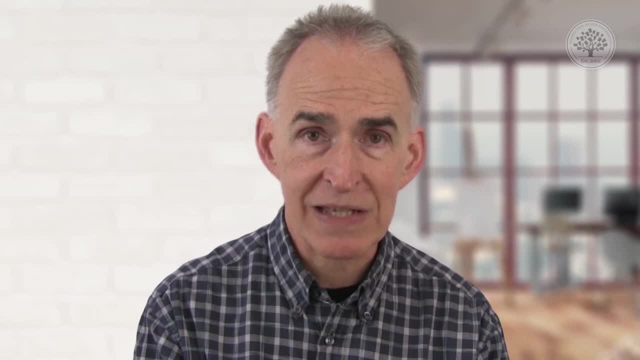 What are they doing before and after interaction with our solutions? fit with their daily routine, for example? And some of this comes from the fact that I have for years been astounded by how little the people developing software solutions know about their users. 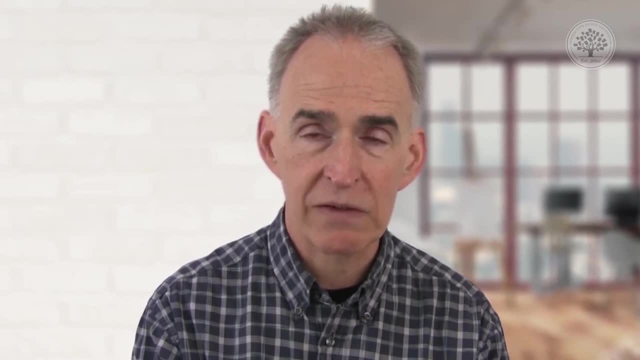 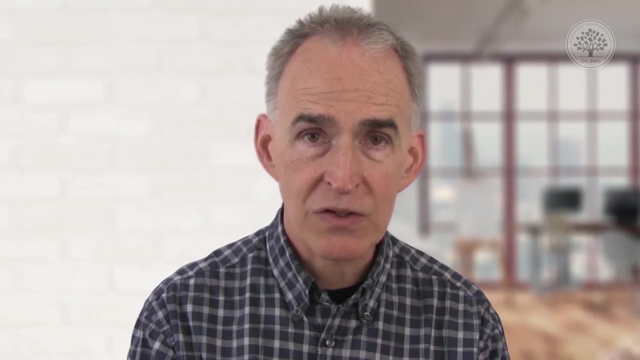 I've been involved in a couple of projects where there was no contact whatever. The development team had never met or seen a user. didn't know what the user was doing was doing immediately prior to entering or receiving data from their system. didn't know what happened to the output data. 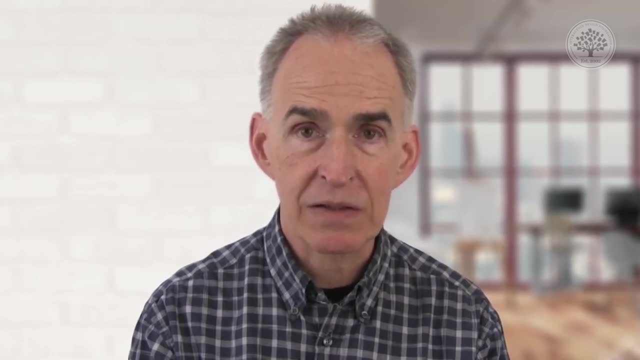 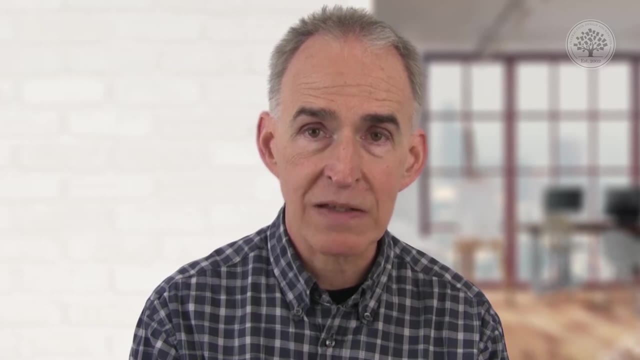 knew almost nothing, So it wasn't surprising that the system, when it was first launched, was almost impossible to use because it didn't actually fit. It was like having a random piece of a jigsaw puzzle in a very well-defined hole that it just did not slip into. 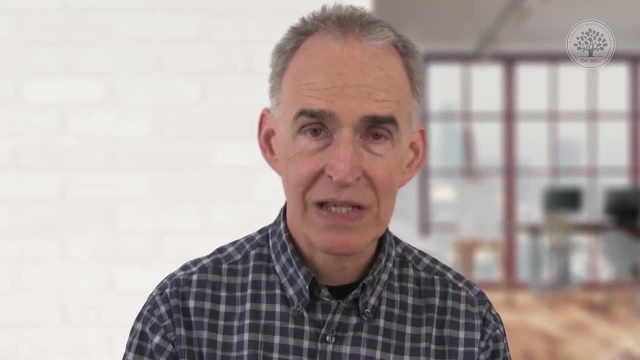 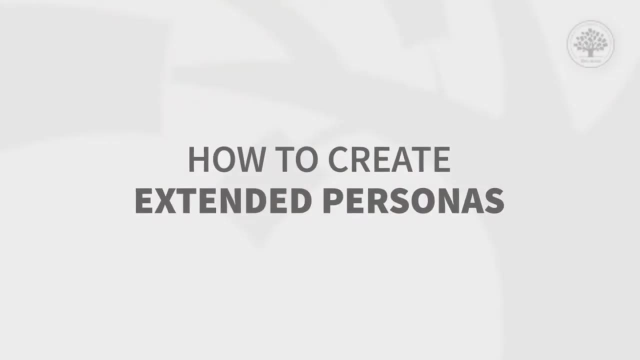 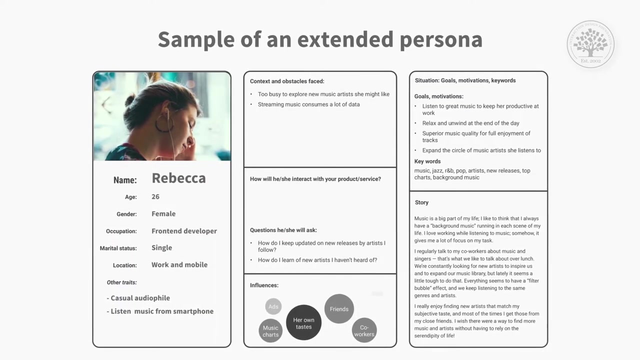 So these are the reasons we're trying to actually make sure that we understand at least something about our user communities, And that's what personas are trying to help us with. Extended personas, you might add lifestyle interests, hobbies, as they apply to their motivations. 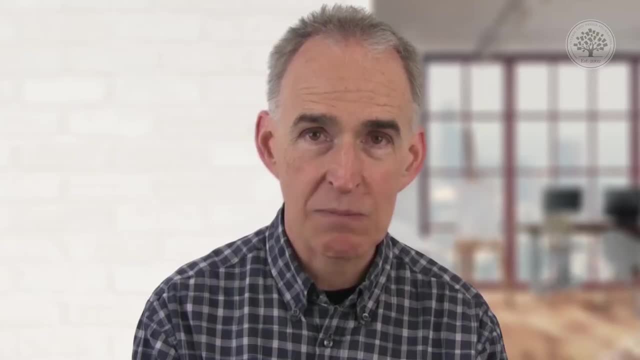 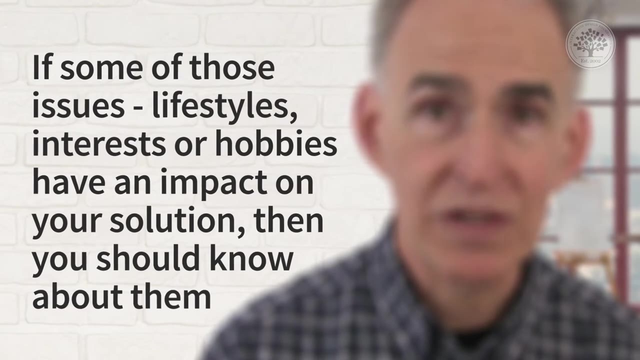 I wouldn't add them just to make the person seem more complete. That isn't absolutely essential, But if some of those issues, lifestyles, interests or hobbies have any impact on your solution, then you should know about them. So keep to the details that are relevant to the problem. 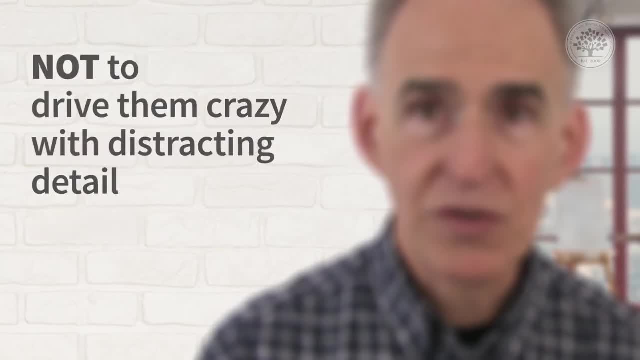 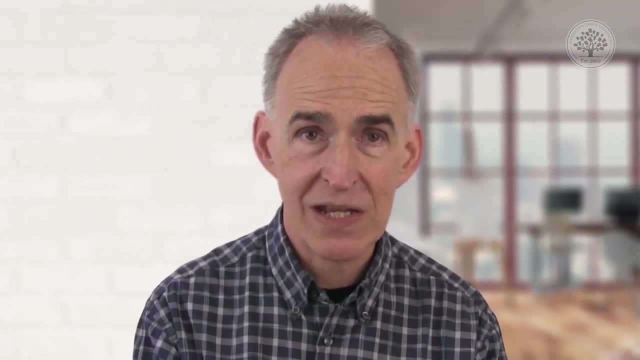 Remember that we want to motivate our team to help our personas, not to drive them crazy with distracting detail, which is one of the complaints you will hear about personas. Certainly, when I've attended conference research papers on the use of personas in teams, often they were not well. 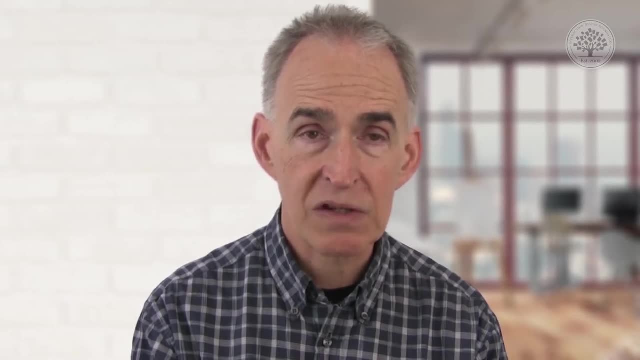 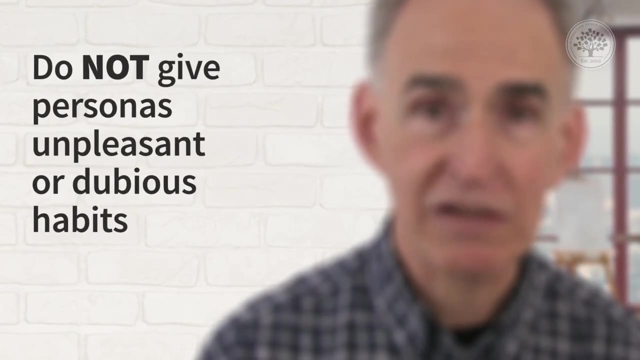 received because there just seemed to be so much of it. the persona specification, Credibility: ensure that the personas are believable and liked as much as possible. Certainly do not give personas unpleasant or dubious habits like being a heavy drinker or a heavy smoker or likes to bet. 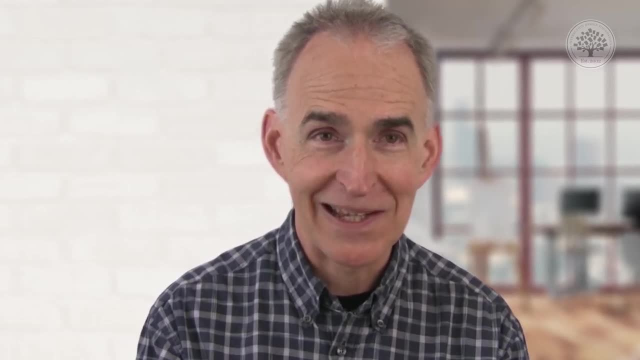 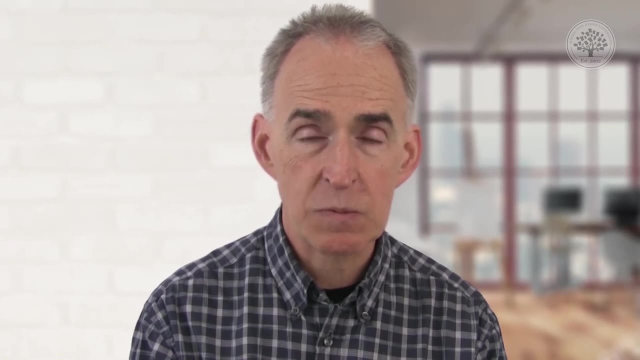 on the horses, unless, of course, you're building a gambling app or something. Change the name, photo and other details until the whole team is comfortable with them. It needs to be a collaborative effort between the user experience people and the people who are going to be using them. 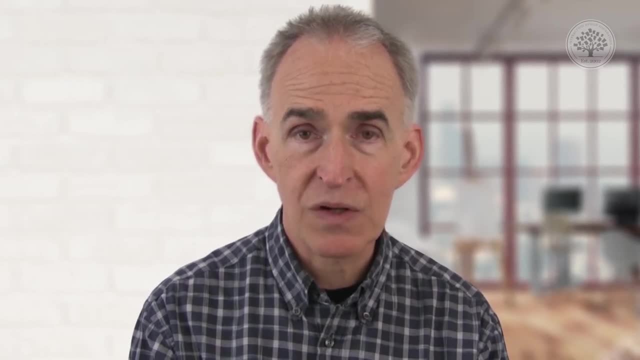 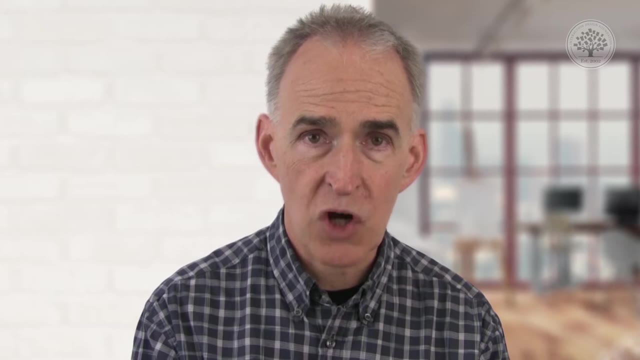 That would be the development team. So the names and the photos are almost entirely arbitrary. If you've done research with a handful of participants, then you'd have a handful of photos. If not, then try to find photos from a stock photo site. 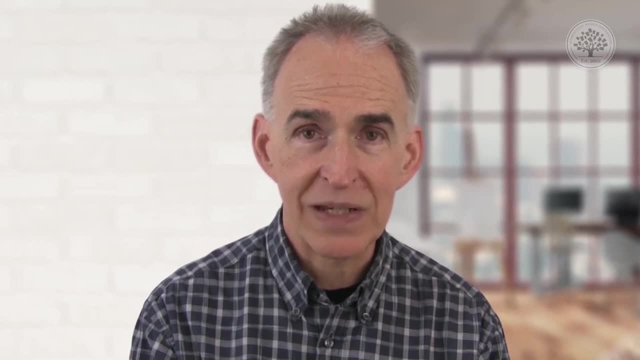 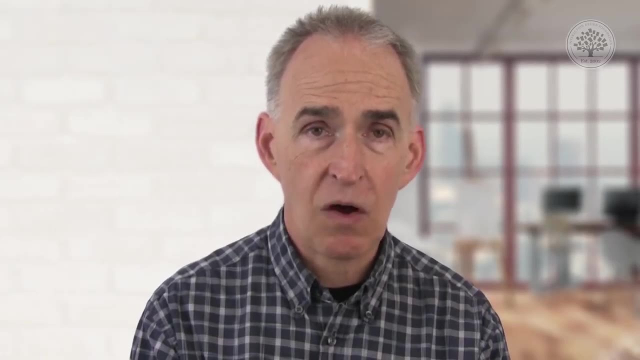 but try to avoid overtly. If not, then try to avoid overtly. If not, then try to avoid overtly, And if not, then try to avoid overtly. So the design team is not necessarily attractive people, because it can be distracting. 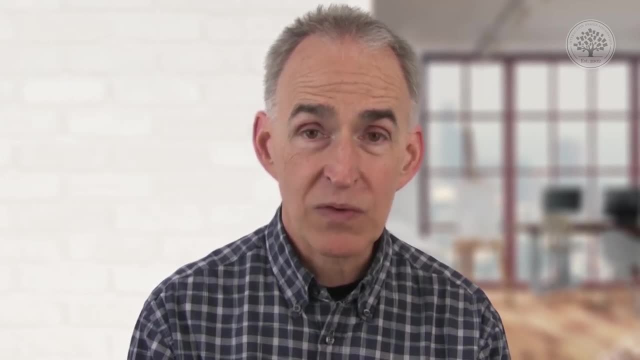 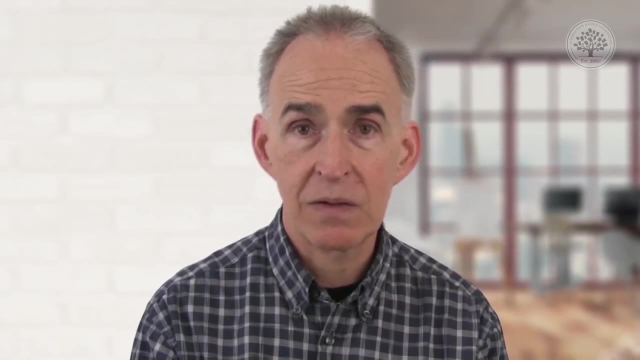 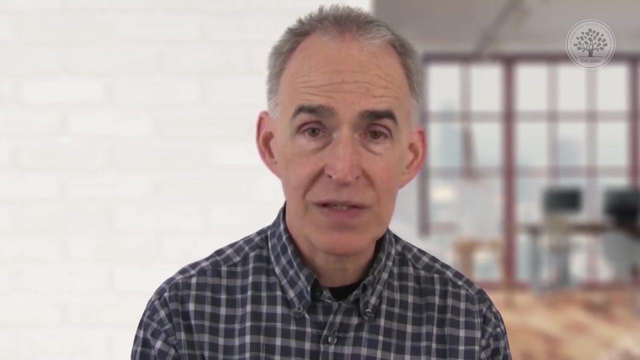 I think in user experience we create often what are referred to as design research personas, or design personas for short. So that's what these things are technically called. We go out and we research these user communities. We decide what behaviors and needs are relevant to us. 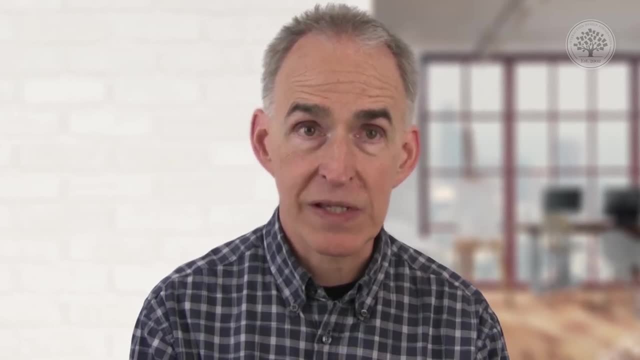 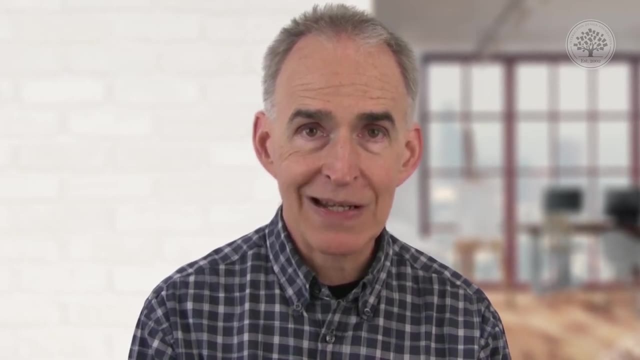 Who are we building this solution for? That's why we want to call them design research personas or design personas. But there are lots of other things that also get tagged with personas, And the most common of those I've come across, particularly in large companies, are market research personas. 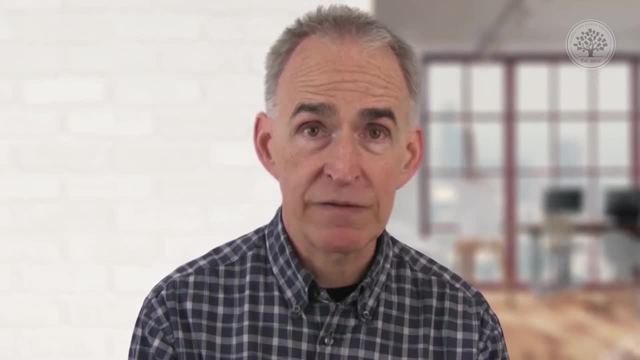 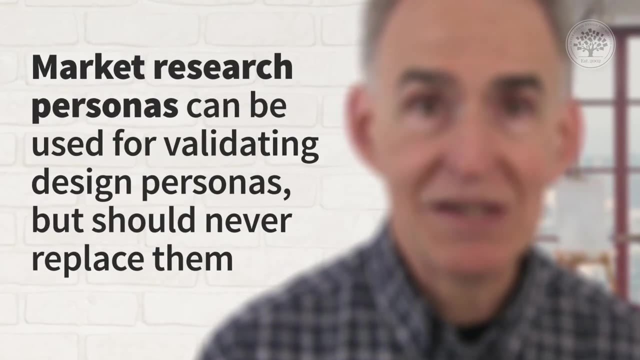 And they're not the same thing is the main problem that we have. So beware that other kinds of personas exist, often based on demographics or market segmentation. These can be used for validating design personas, but should never replace them. There is little point in trying to reuse. 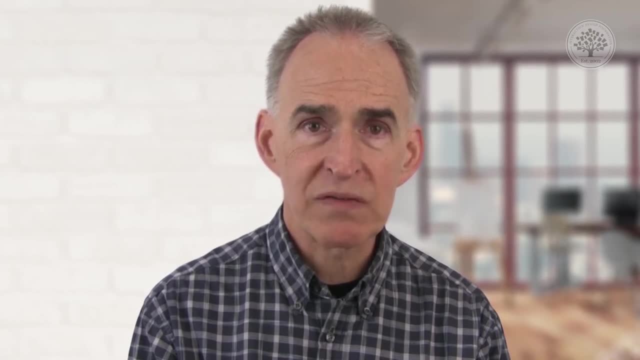 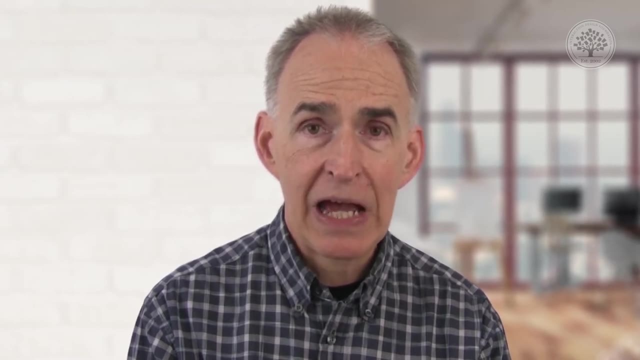 personas for different projects as well, unless the same goals, motivations and behaviors are relevant. And I've come across this whole approach in one particular vertical market in the UK and that is mobile phone service providers- that they have all got marketing personas based on age ranges. 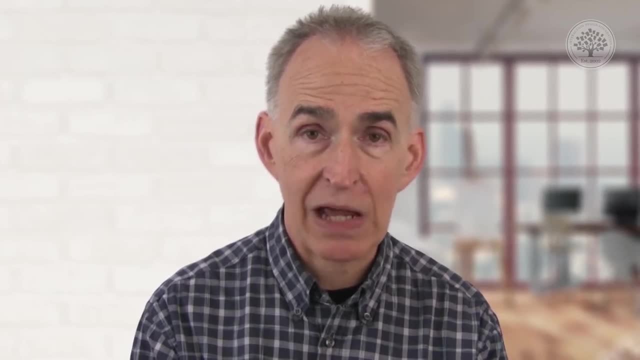 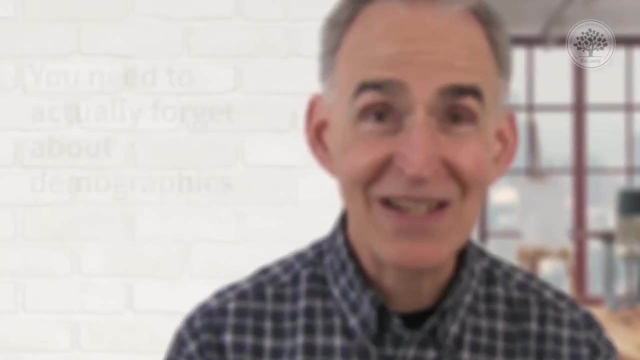 And they then attach labels to these age ranges to suggest how these people behave and what they need from our services, which, just to be honest, cannot really be true. You need to actually forget about the demographics. There will be some age-related behaviors, no doubt. 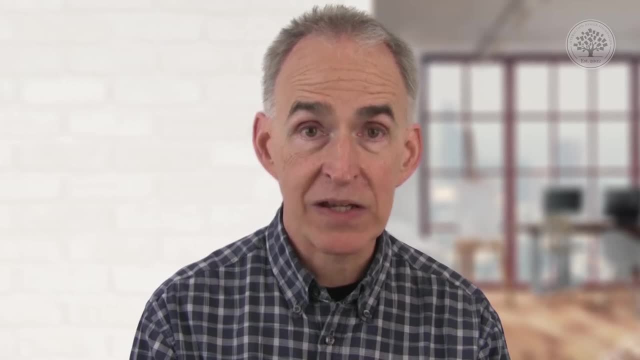 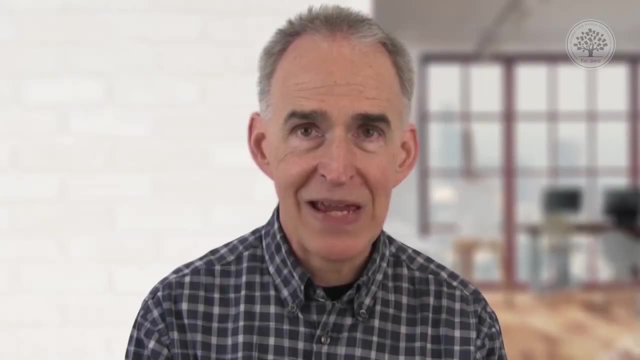 but they shouldn't be the motivating factors in the design of an interactive system, which is, after all, what we're trying to achieve. The main thing is that, predominantly, you have one or two primary personas. If you've got a project- and I've had people- 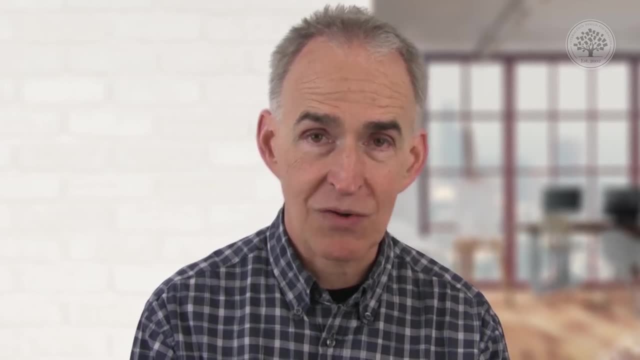 kind of come up to me almost in a boasting tone, saying our project has got 20 to 30 personas, And I'd say, oh really, How is that? They'd say, well, it's a hospital, It's a hospital system. 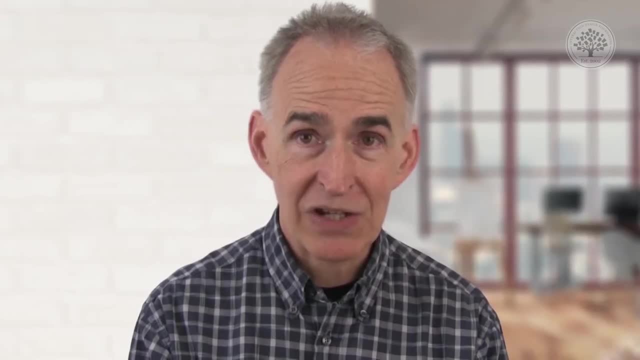 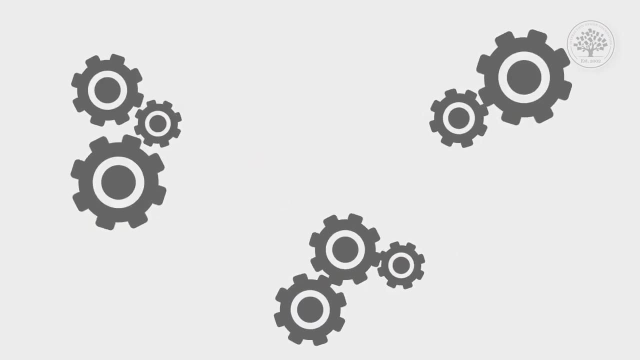 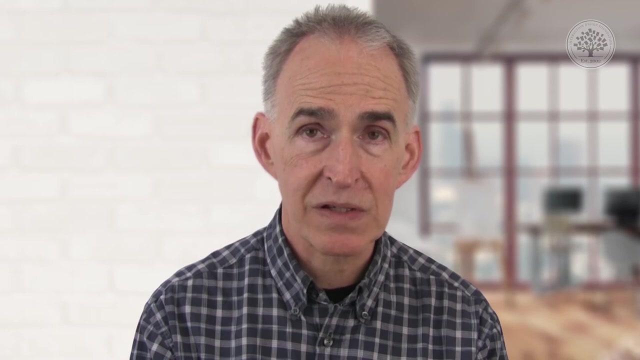 And the thing is it's a very big system And what you need to make it agile and to make these things work effectively is to split the system into parts, So you may well have some small number of primary personas that apply throughout, but in many cases you're going to have primary personas. 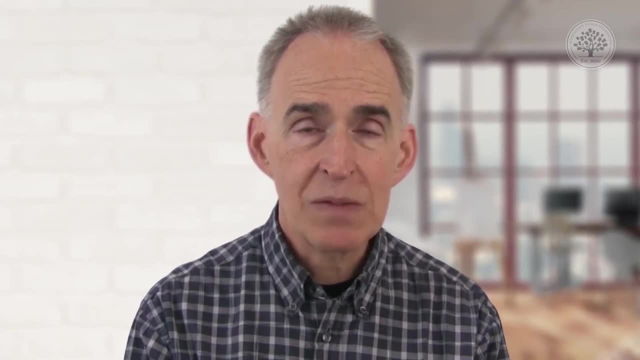 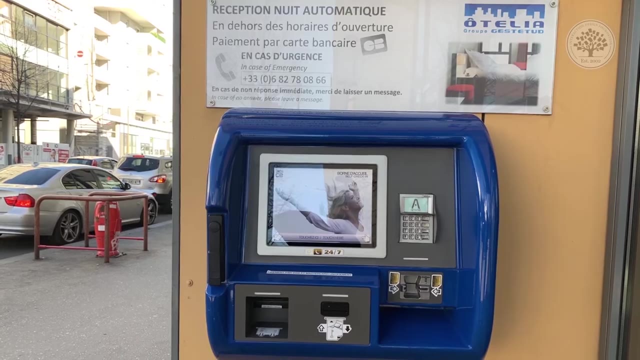 that are specific to that kind of system or that part of the system. So let me give you some very simple examples. The one that I like to use is a hotel self-check-in. When I started writing about hotel self-check-ins, there were none in existence. 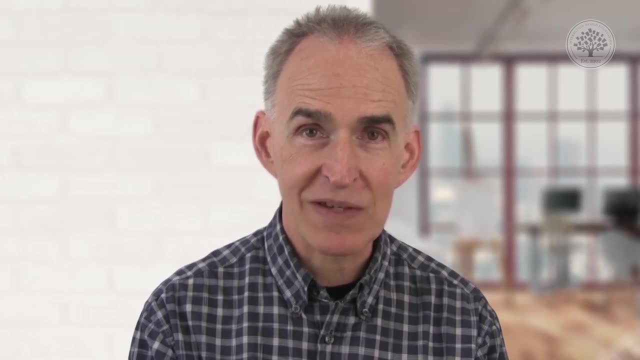 And now I do come across them, funnily enough, in hotels that have got receptionists, but all they do then is to refer you to the self-check-in in front of the reception. I was motivated for this example by checking in at a conference. 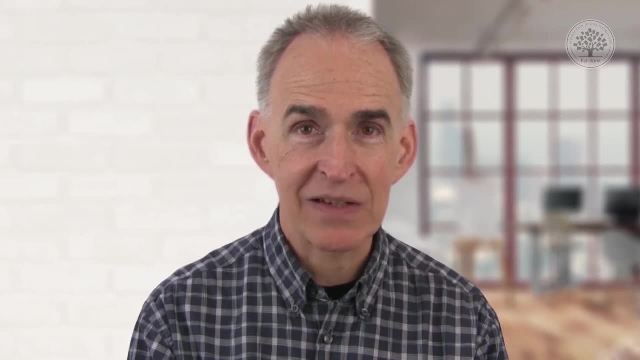 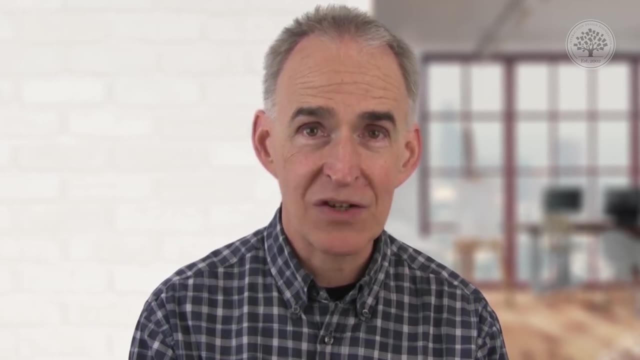 hotel. on one occasion I actually got in pretty easily. I think it was a 20 or 30-minute process. But the next day I was walking through a reception And the queue, the line of people waiting to check into this hotel. 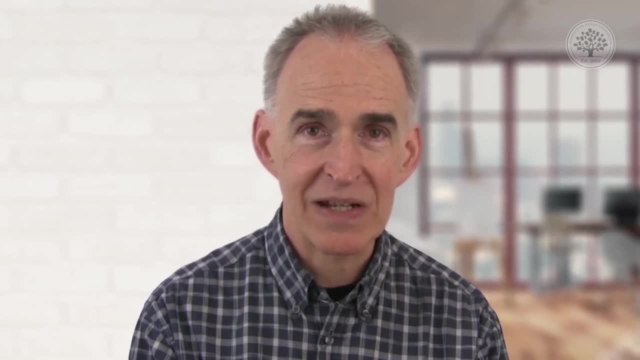 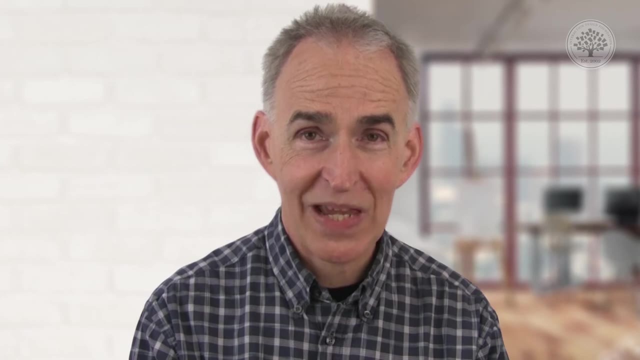 went around the block. It was just utterly amazing. There must have been 200 or 300 people waiting to get in. So it occurred to me: well, why don't we just have some self-check-ins, like we do at airports, And, of course, self-check-in at airports? 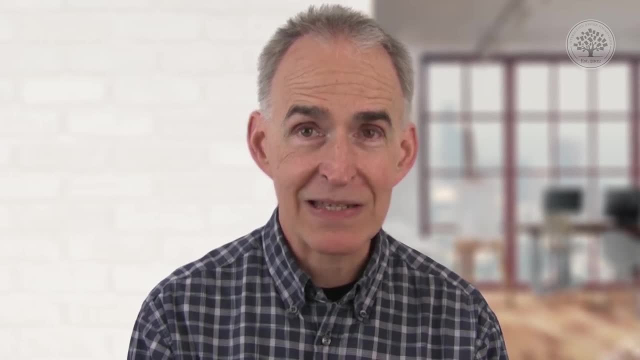 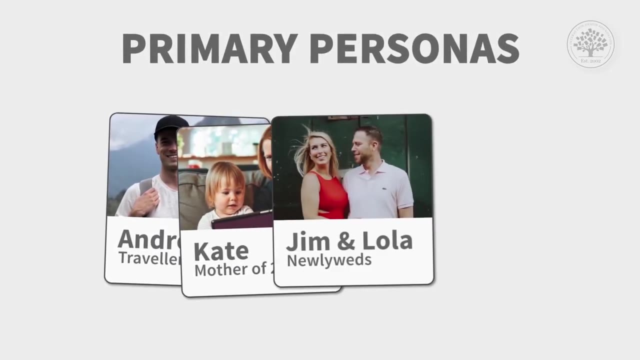 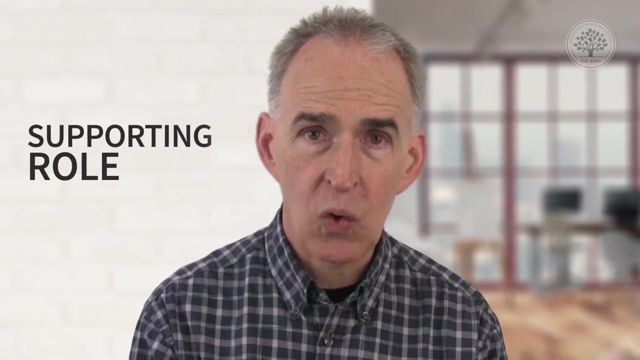 is entirely bog standard these days. It's what everyone does. So, for example, the primary persona of a hotel self-check-in service must be the customer checking in. It makes no sense for it to be otherwise. A secondary persona would be someone who is acting in a supporting role inside that system. 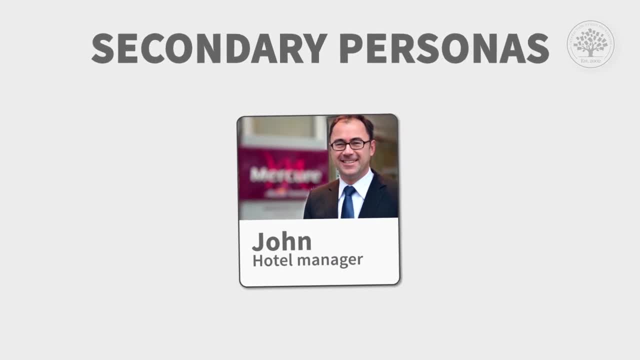 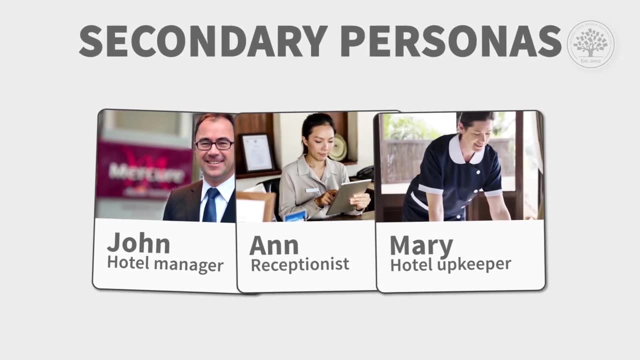 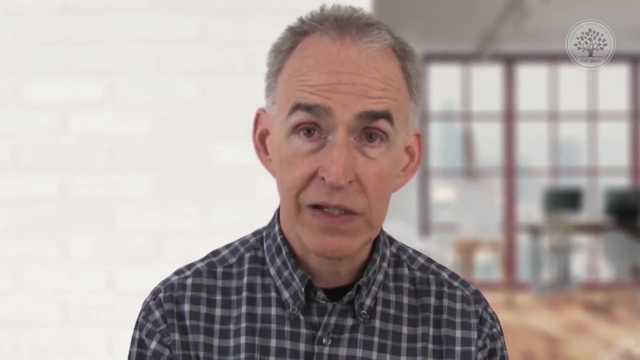 So a secondary persona might be a hotel manager or a receptionist or somebody who's responsible for the upkeep of the hotel, for example. So these are all secondary roles. They're not the people for whom we are building the system. They are people who are involved in the system. 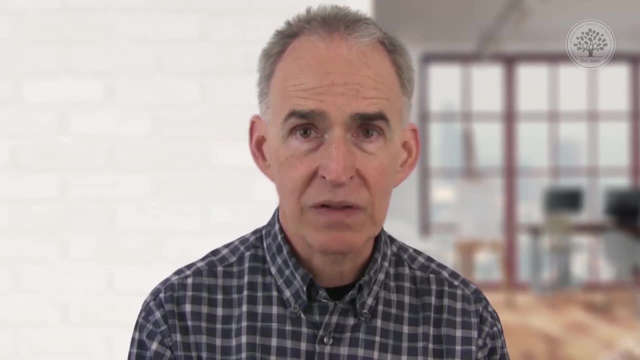 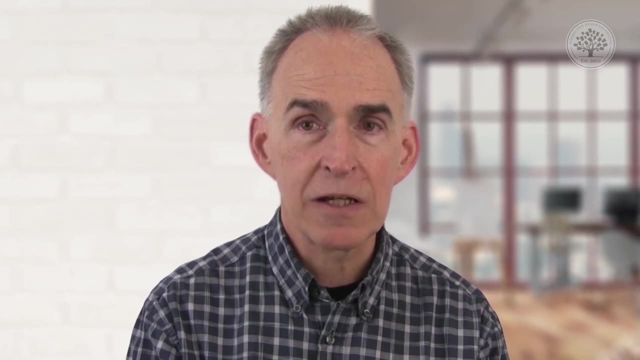 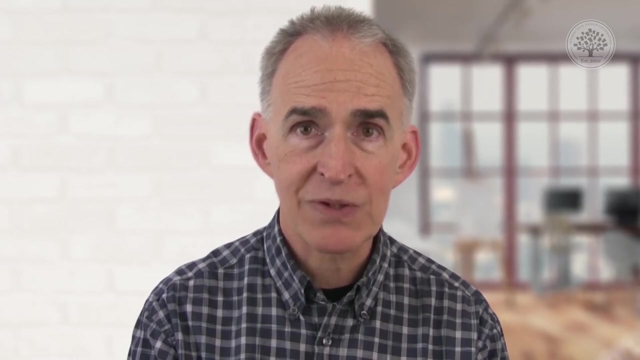 and often in a backroom kind of interaction. These are people that primary personas rarely see or even know about. So it's a difference between the primary roles in a stage production and just extras, people with non-speaking parts. That is kind of the difference between primary and secondary. 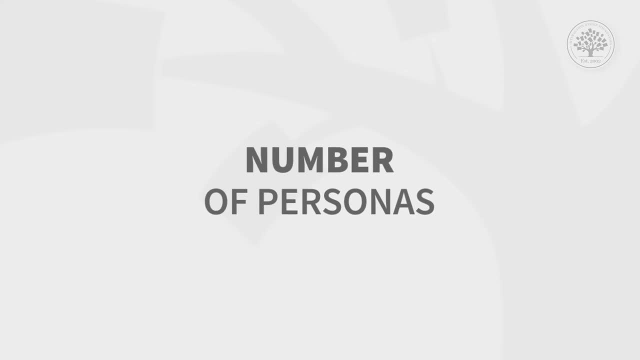 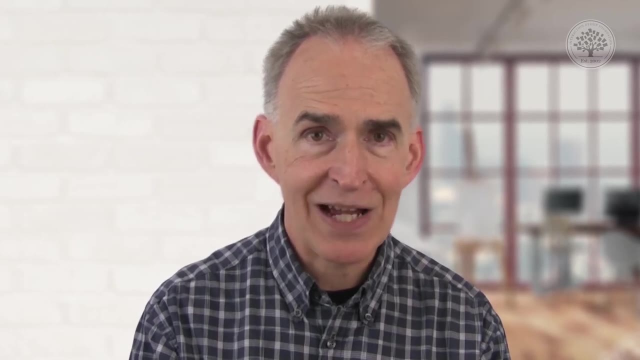 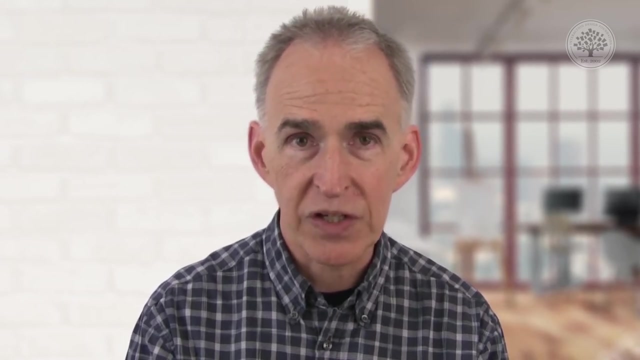 personas. A lot of systems may have only one persona. This is the person that we're building this particular product for, And you can have all kinds of philosophical arguments about whether you're building a Swiss army knife solution or whether you're building a carving knife solution. 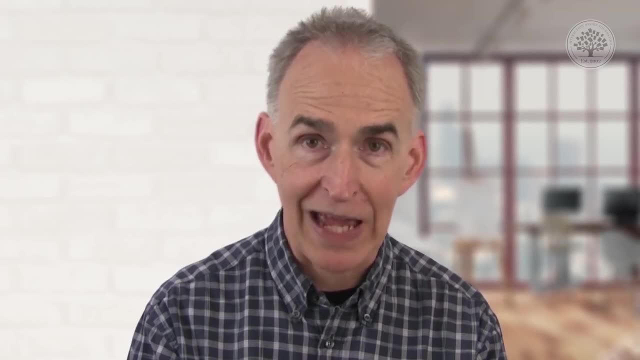 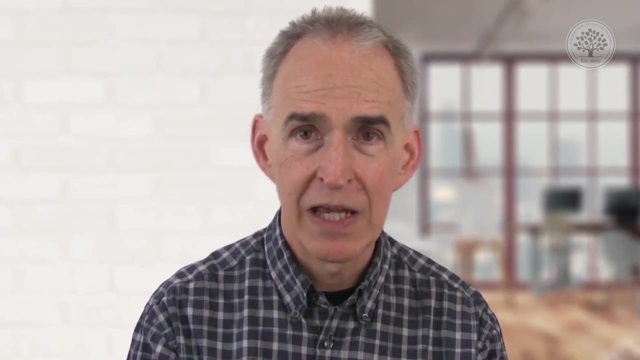 One is very good at one thing: Carving knives are very good at carving. Swiss army knives are very good, but in a fairly different kind of way, at all kinds of things. But they're not all that easy to use. So it's up to you. 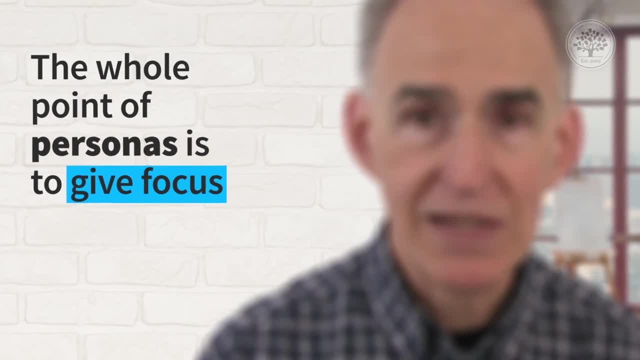 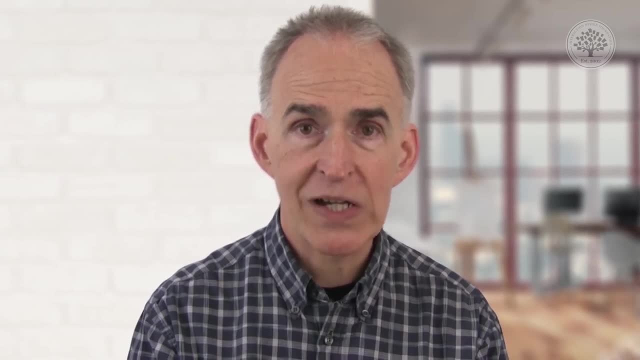 The whole point of personas is to try to give focus. So these are our customers, other people who do not fall into the definition or the descriptions of our personas. It's fine if they find our system easy to use, But unless we can actually identify some clear purpose, 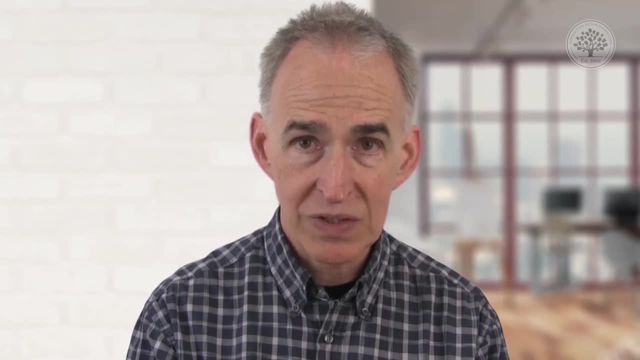 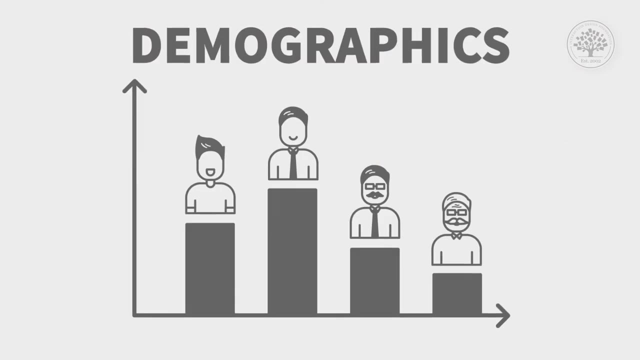 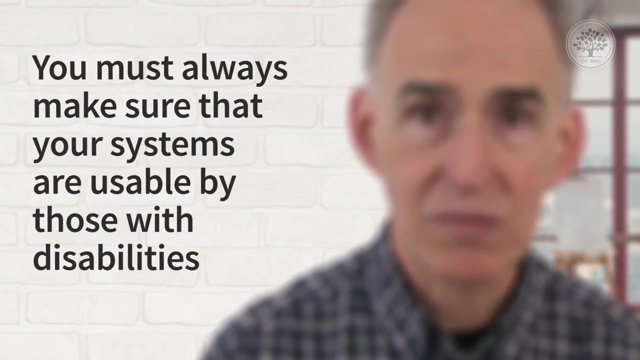 in adapting the system to be more inclusive, then we would deliberately not pay much attention to their particular requirements. Now, things like accessibility and the age ranges of users. they fall out outside the whole persona mechanism. You must always make sure that your systems are. 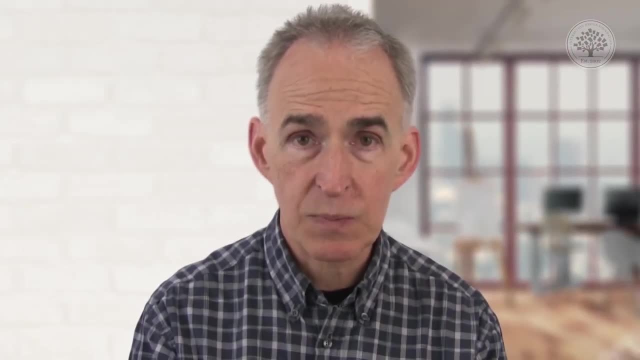 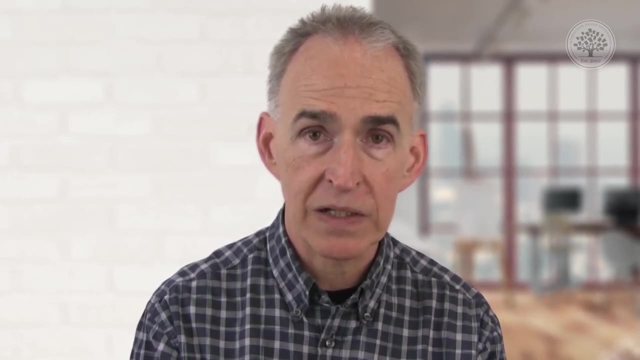 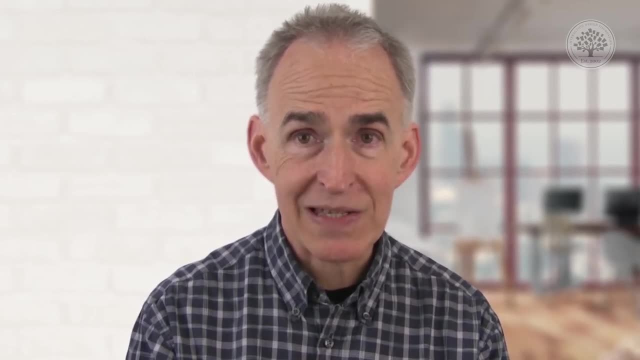 I think that's a good point. I think that's a good point. I think that's a good point. He deliberately includes a disabled persona, But that really ought not to be necessary. But if that works for you, then that's absolutely fine too. 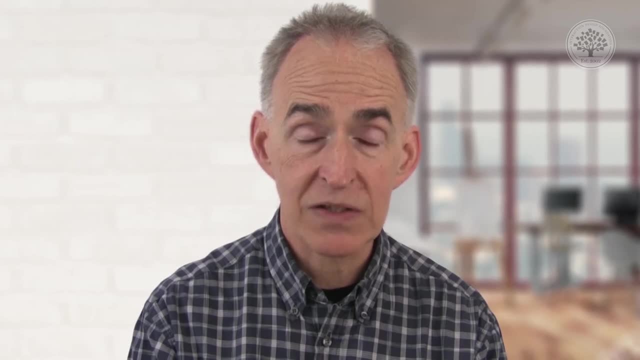 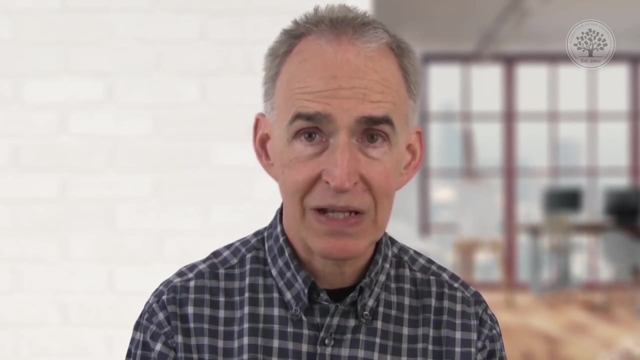 It's certainly. I can see it being important when working with teams that don't have much experience, So you must make sure that your solutions work for a broad range of people in terms of accessibility and age issues, But otherwise we want to be very focused. 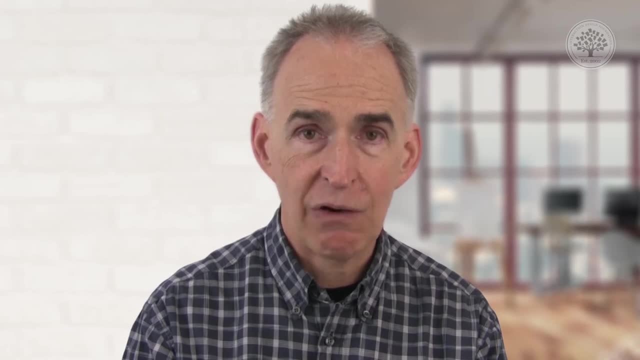 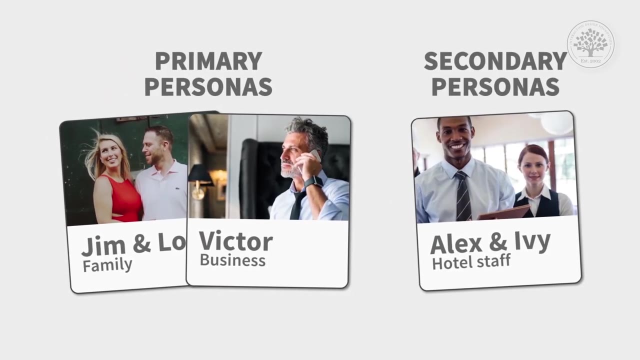 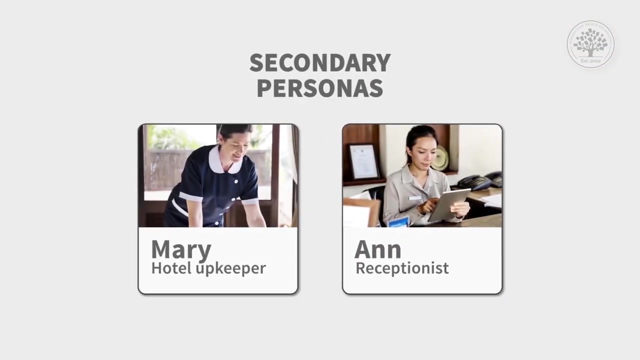 on the specific behaviors and needs of our primary personas. So we stick to small numbers to maximize the number empathy and we consider splitting larger projects, as I was discussing for the hospital example. but for example, a hotel check-in system could be split into front desk and housekeeping projects with separate personas. so those could be. 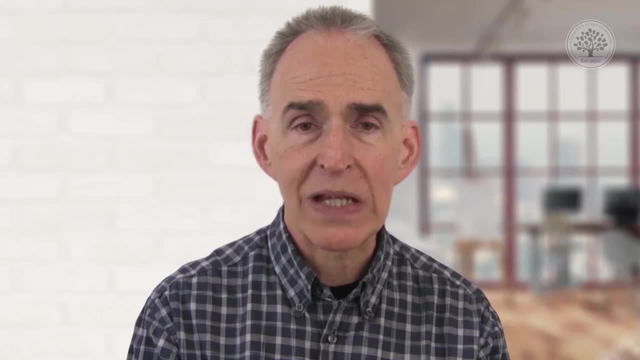 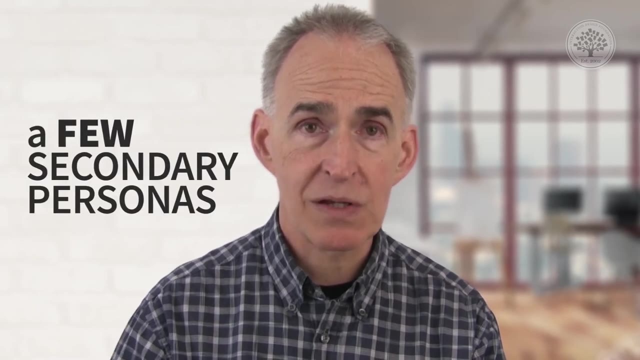 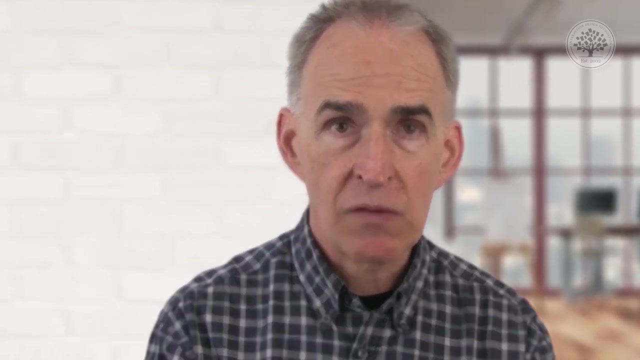 two smaller agile projects and there is no magic number. but, like I have been saying, one or two primary personas is perhaps the most common, with maybe a few secondary personas thrown in as well. personas get used in all sorts of places. obviously, the main focus is in design. so who are we building this product for what? how should the 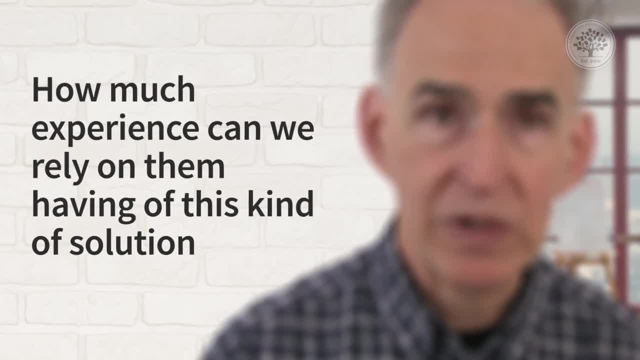 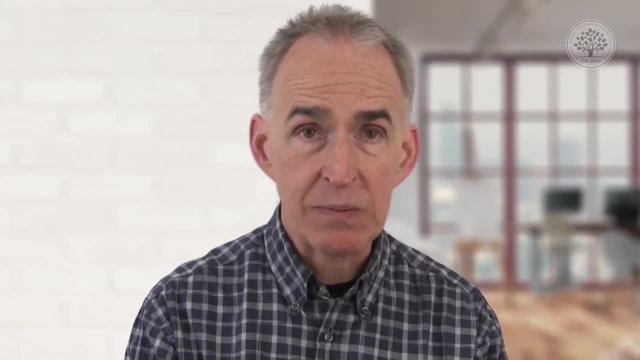 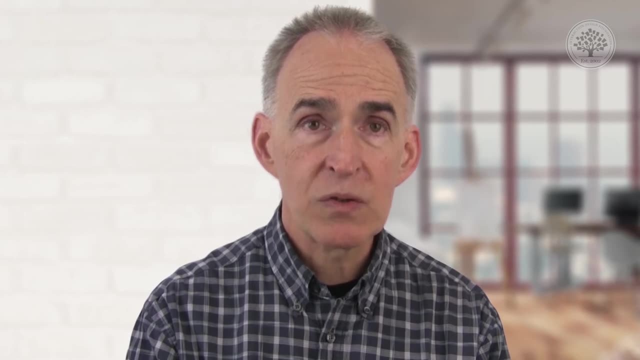 interactions take place, how much experience can we rely on them having of this kind of solution, and so forth. we will have to recruit these people. we want to do research with them, perhaps continuing research over several lifecycles of the system. we want to recruit people for usability testing in. 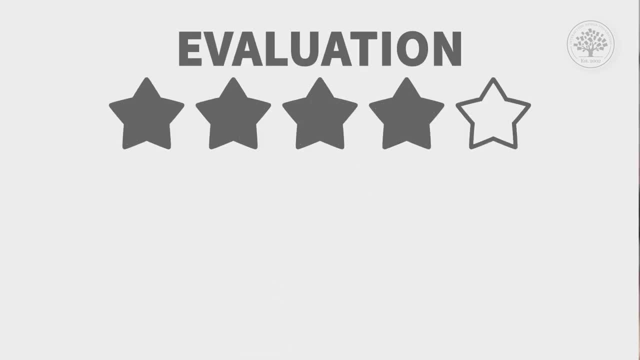 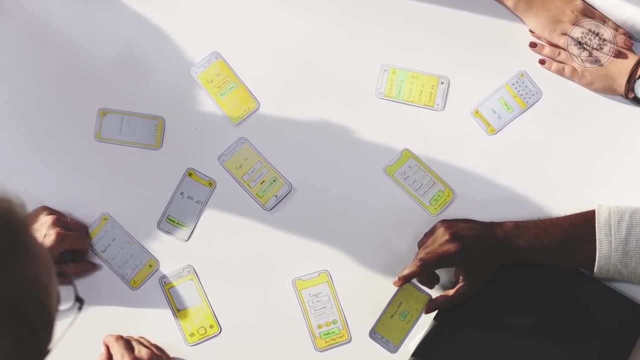 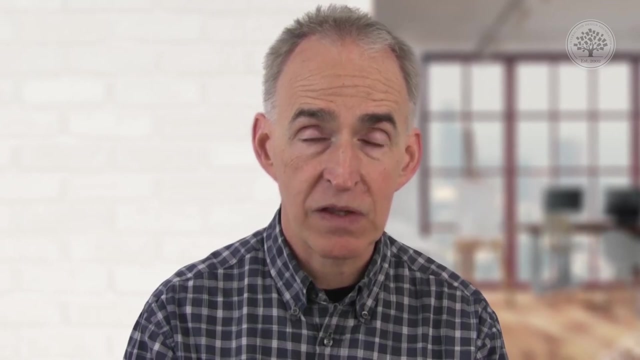 user evaluation, usability evaluation in general, not just running them through early beta releases of the software we might want to be testing with paper prototypes. we might be wanting to show them just wireframes and talking to them about the layout and their understanding of the different components of the page. those sorts of 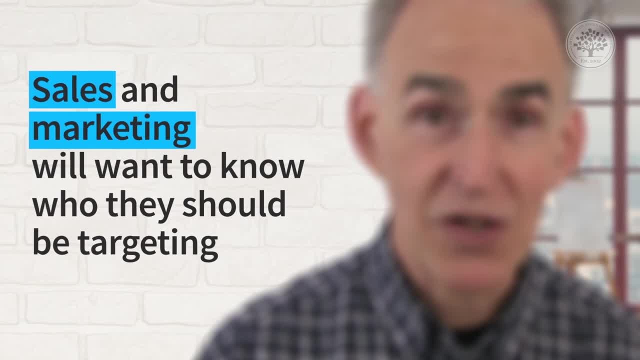 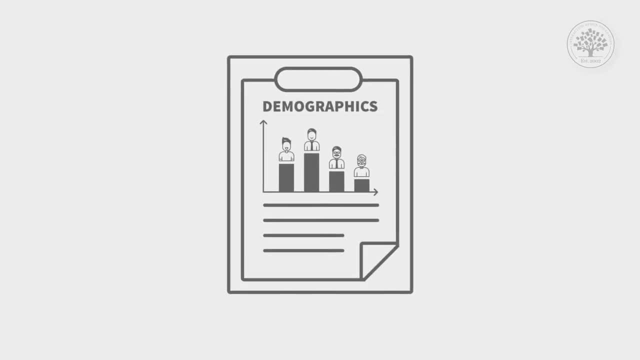 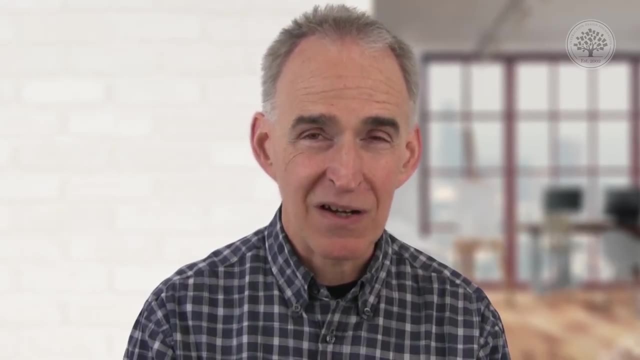 issues, sales and marketing will want to know who they should be targeting in terms of what this system does and for whom, and remember that you will need to describe the demographics and the filtering questions for your personas to a recruiter. so, when you're recruiting authors, what is it about, Arthur, that? 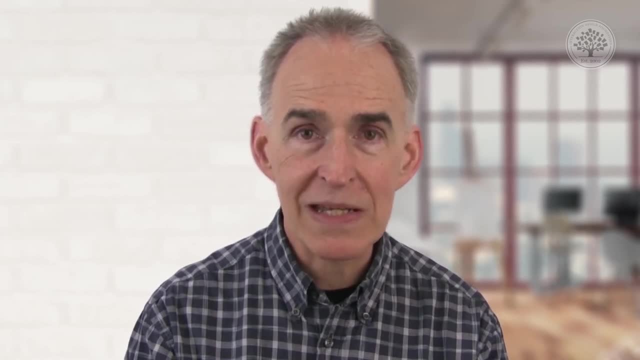 makes him your persona. it needs to be something that he wants or needs, or you're hoping that he wants or needs, needs, a solution to a problem. so what is that problem? so you need to actually talk to your recruiters about filtering questions. what are you going to ask potential authors? that's going to help. 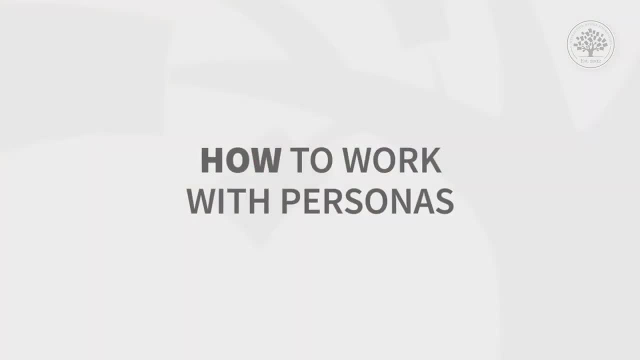 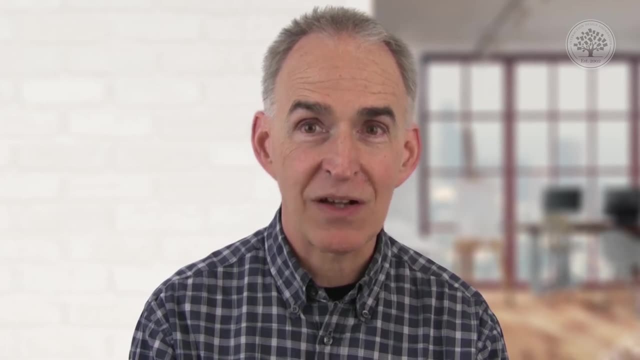 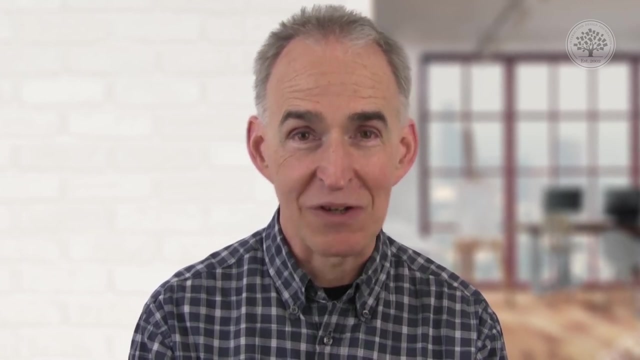 you to decide whether this person is really an author- you now this is quite an interesting area, and it may depend a lot on how enthusiastic your team is about personas, if you've done your job right, if you've sold personas, or if your team is already quite familiar and quite enthusiastic. 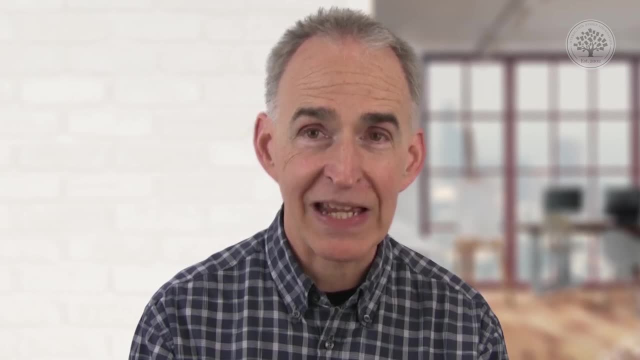 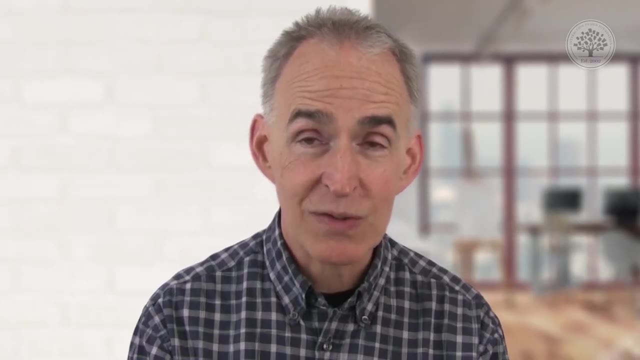 about personas, then you might do some really fun things, like getting mugs and coasters printed with, maybe, the face of the persona on one side and some of their relevant details with respect to your system on the other side. ditto with mugs, maybe even t-shirts, and one thing that I was-